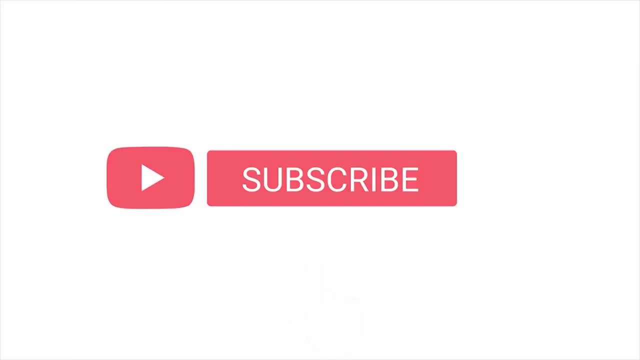 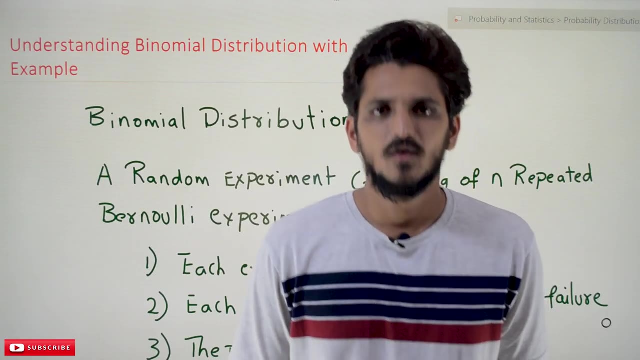 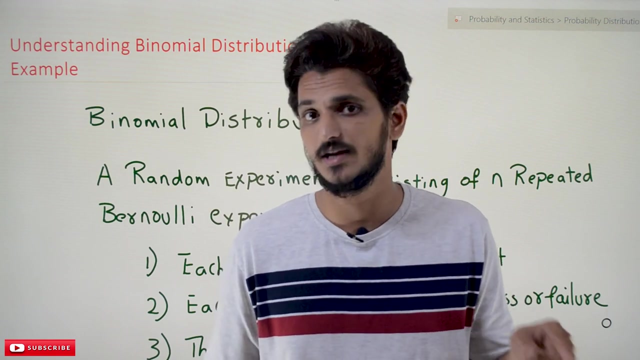 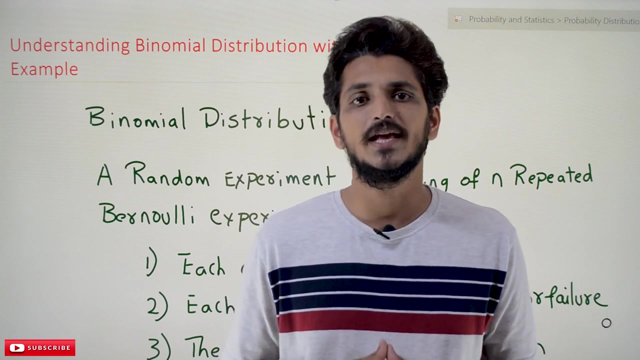 Hi, welcome to Learning Monkey. I am Raghu here In this class we'll discuss about binomial distribution. In our last class we clearly discussed about what's Bernoulli distribution means. Please watch that class and come back here. The link for the playlist is provided in the description below. 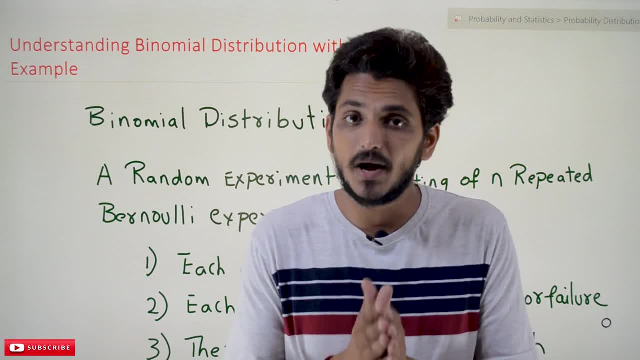 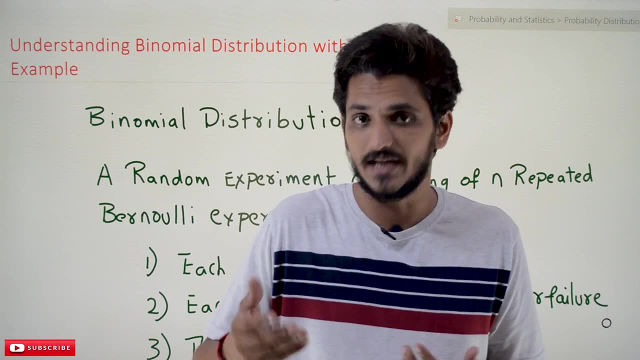 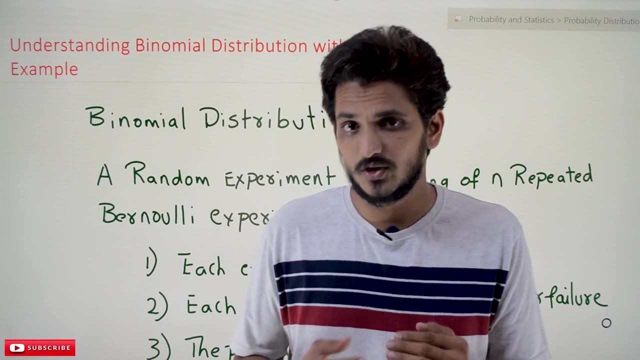 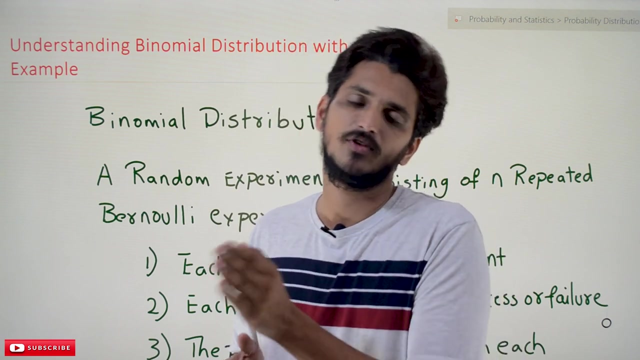 Coming to today's class, binomial distribution is very much used in our real-life examples. So how we are going to use in our real-life examples, in data analysis examples, we will discuss in our next coming classes. So in this class we are going to understand when we need to apply binomial distribution and what is the probability mass function for binomial distribution with simple coin example. 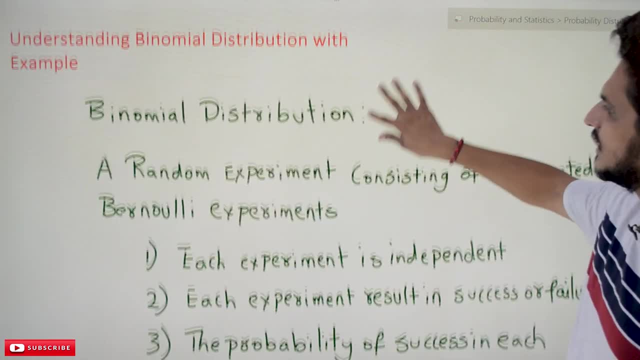 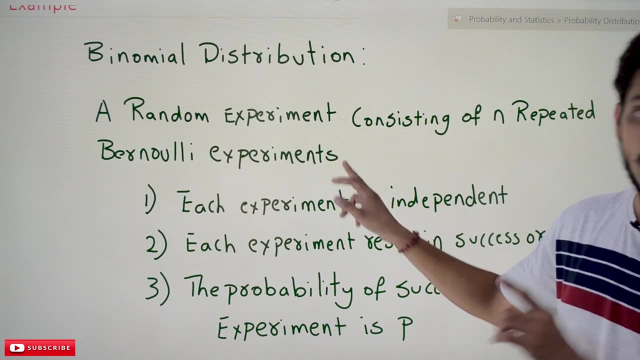 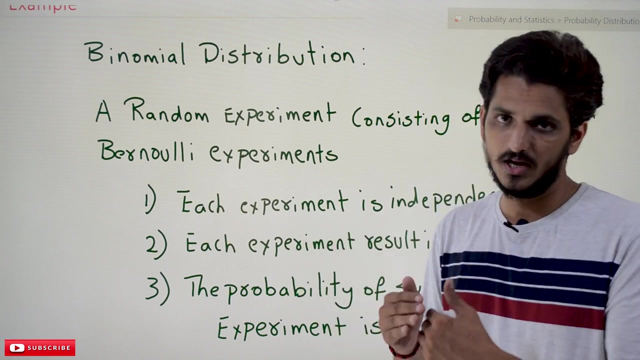 Coming to today's class we are going to discuss about what's Bernoulli distribution means Coming to today's class. binomial distribution is a random experiment consisting of n repeated Bernoulli experiments. In our last class, when we discussed about Bernoulli experiment, it should have only two outcomes: either success or failure. 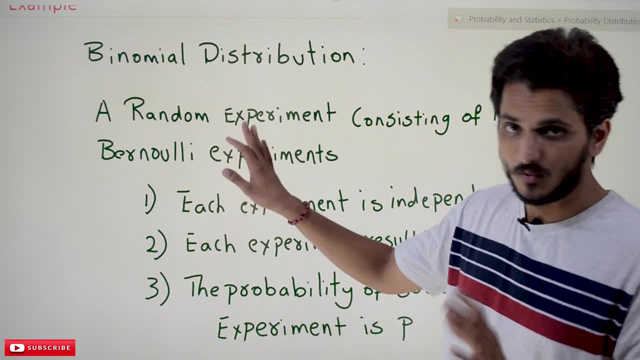 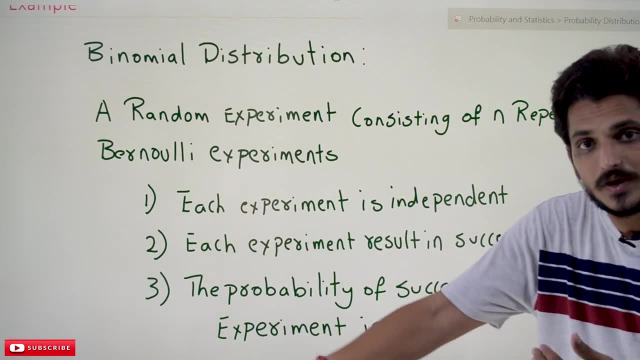 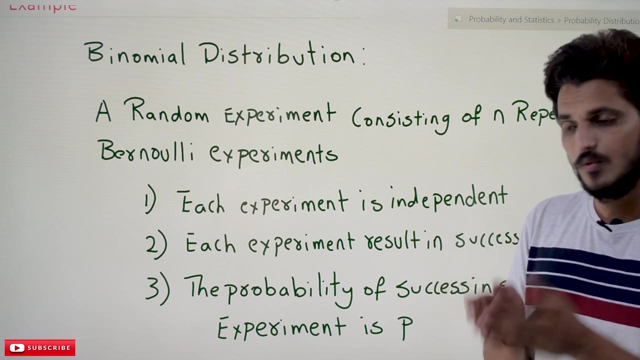 Then we say it as Bernoulli experiment. So what we are saying is a random experiment consisting of n repeated Bernoulli experiments. Means tossing a coin Is a Bernoulli experiment. If you consider head as success, we call it as head is success, tail means failure. 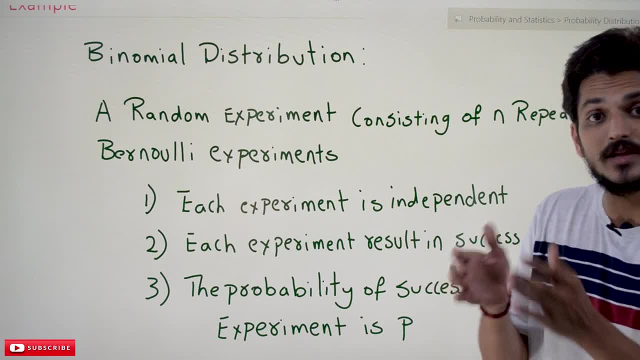 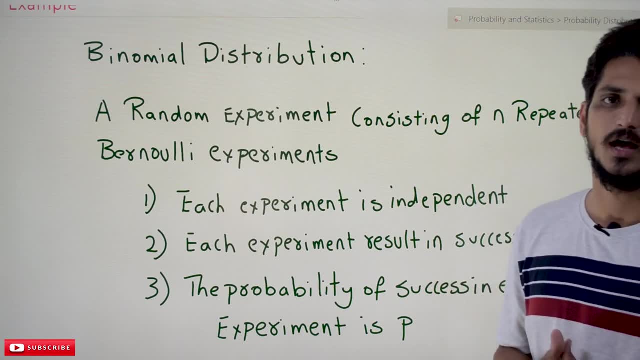 So it is a Bernoulli experiment. If you repeat this experiment for n times, then we can make it as binomial distribution, But it has to follow some conditions. What's these conditions? Let's try to understand. Each experiment is independent. 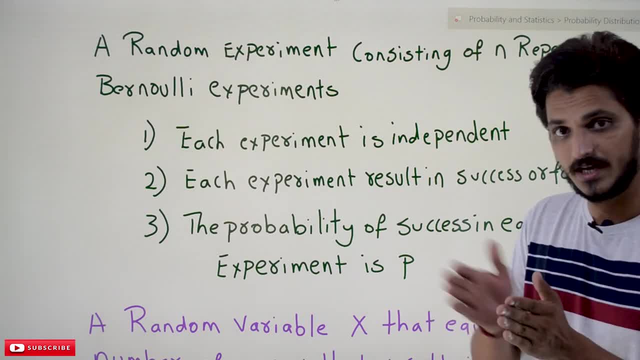 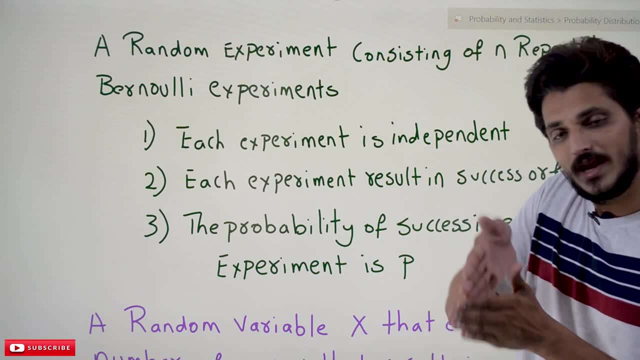 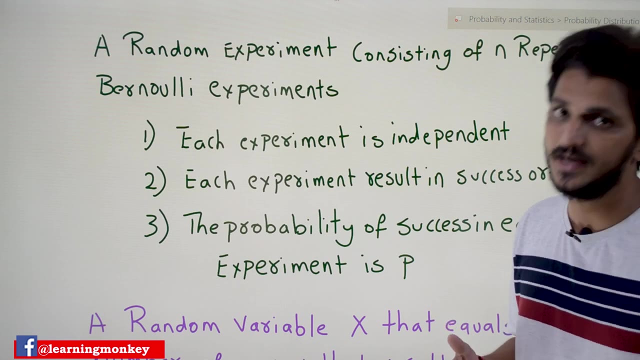 Yes, tossing a coin is an independent event. Second time Because means independent event. means we already discussed previously in our examples: Independent event means one event occurring of one event should not affect the probability of the second event. Those two events are we call it as independent events. 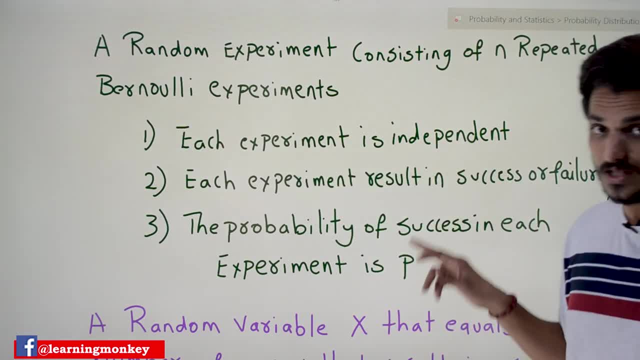 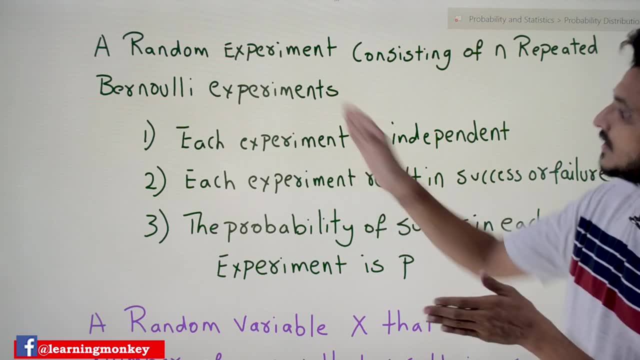 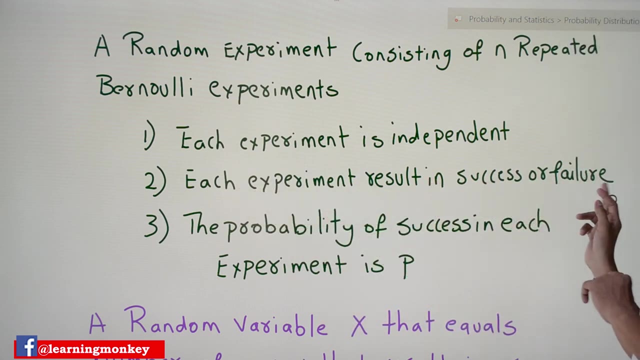 So each experiment is independent. This is very, very important to remember this point. in binomial distribution, Each experiment, each Bernoulli experiment is independent of each other. Each experiment, Each experiment result in success or failure. Because we are following Bernoulli experiments, it will have only two outcomes. 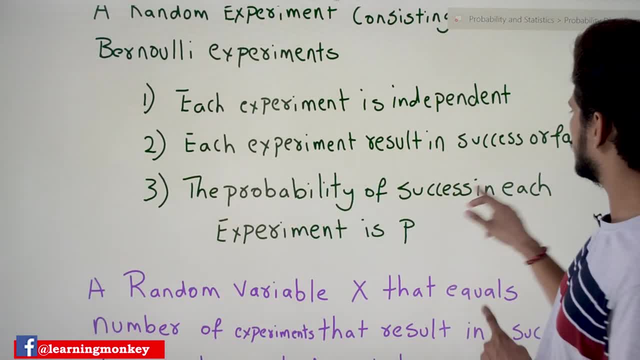 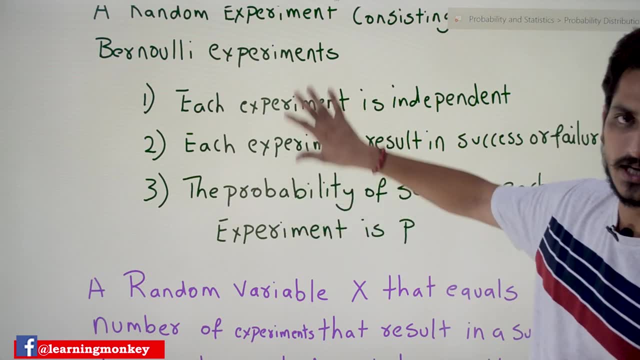 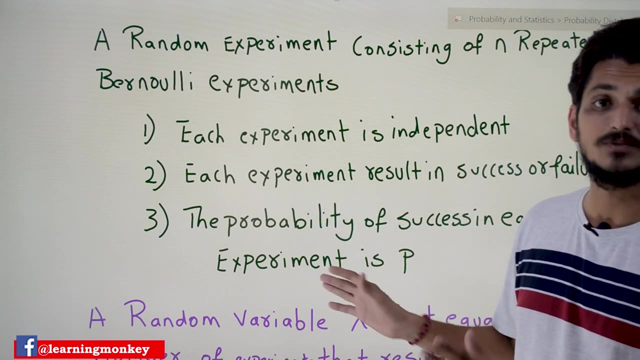 It is success or failure. Probability of success in each experiment is P. These are the points you have to satisfy, Then we can. we can. if your experiment consisting of these conditions, then we can make it as binomial distribution. Until now we did not understand what's binomial distribution. 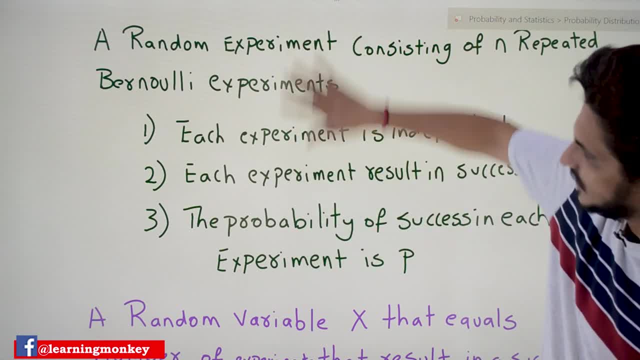 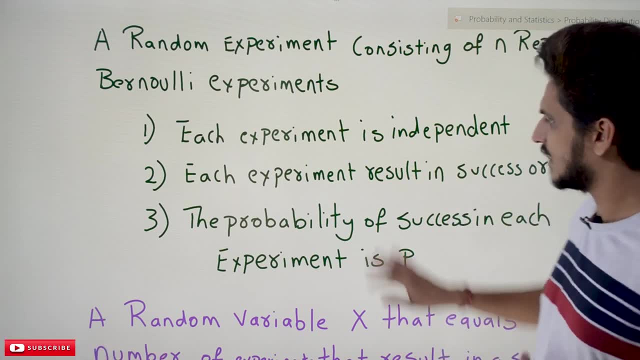 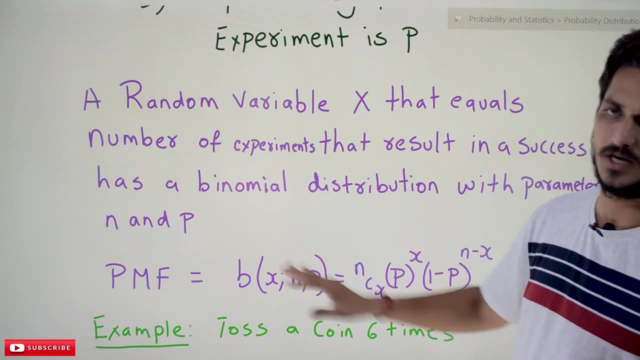 What's binomial distribution? If your experiment follows these conditions, then we can apply binomial distribution. That is the point you have to understand. Now, coming to the probability mass function, then we will. with example, we are going to understand binomial distribution. 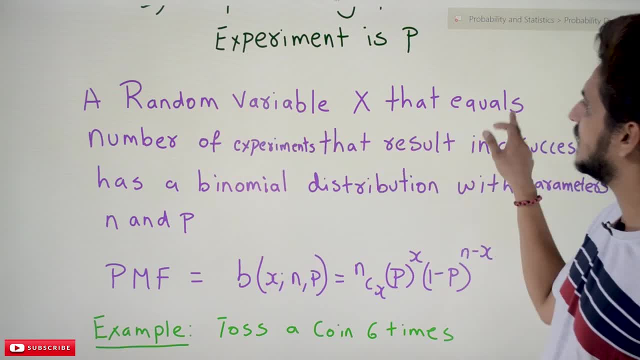 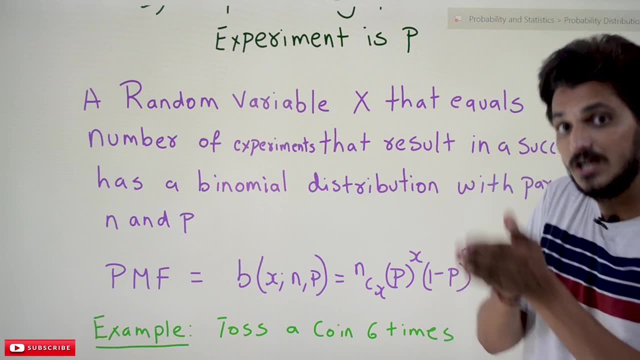 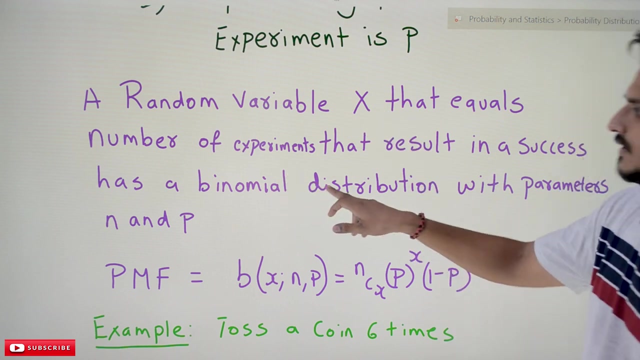 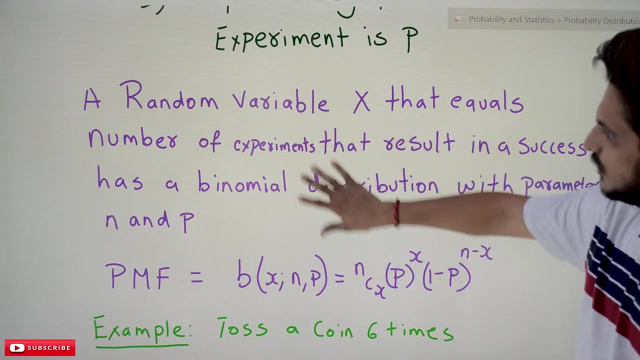 A random variable, x that equals number of experiments that result in a success. Number of experiments that result in a success. That random variable has a binomial distribution with parameters n and p, So we are going to understand this statement at the end of the class. 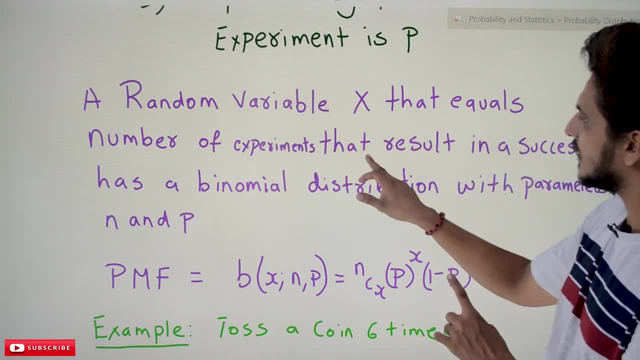 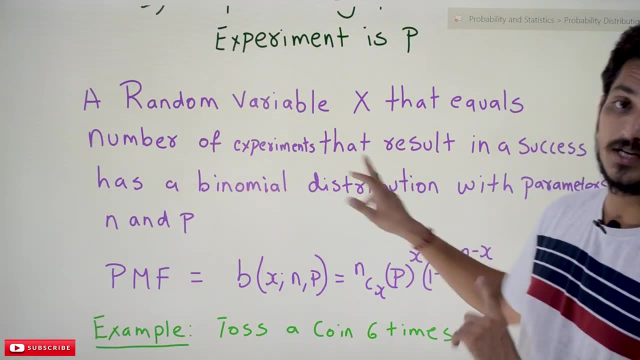 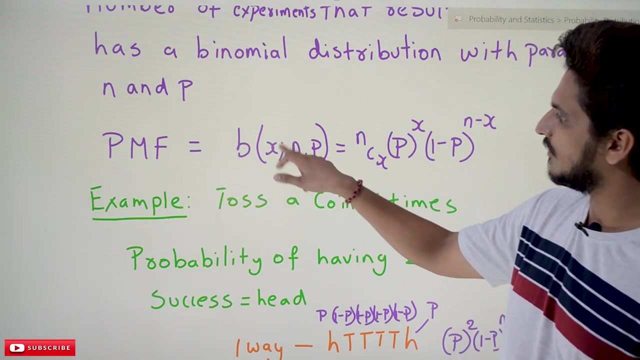 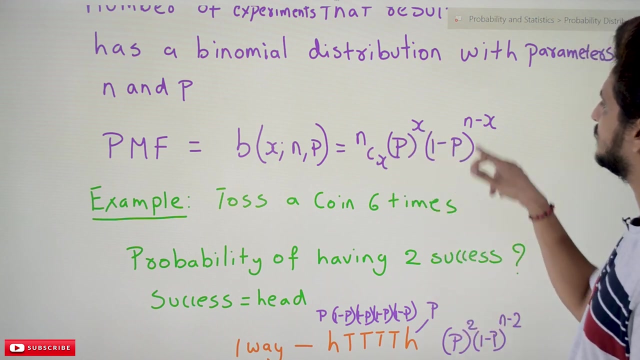 For just now, remember x, that equals number of experiments that result in success. Then we can make it as binomial distribution with parameters n and p, So probability, So probability, mass function is given as binomial of x, comma, n, comma p is given as ncx, p power, x multiplied by 1 minus p, power n minus x. 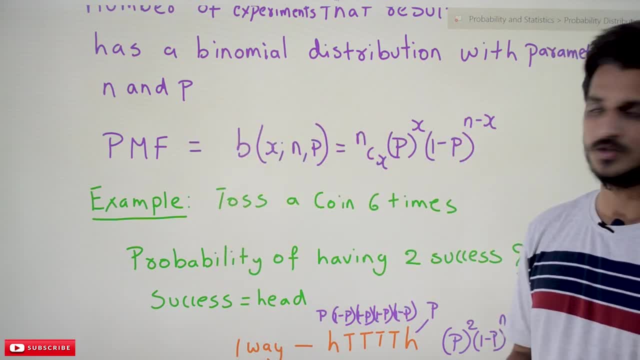 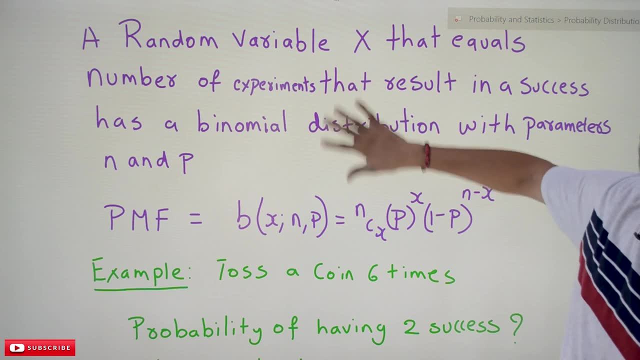 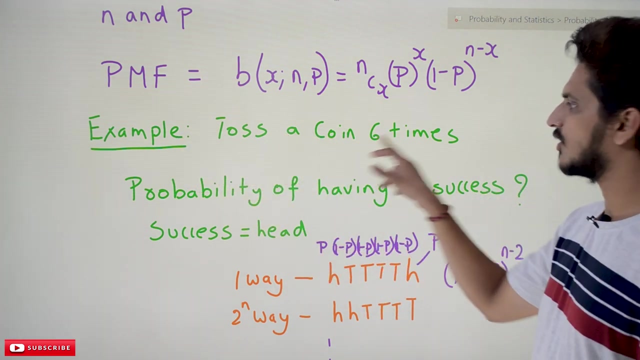 This is what probability mass function for a binomial distribution. First we have to understand how we got this probability mass function. Then we are going to understand this statement. Okay, So let's take an example and understand probability mass function. Example: toss a coin 6 times. 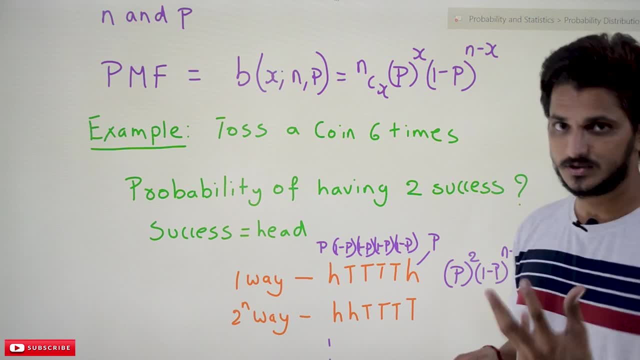 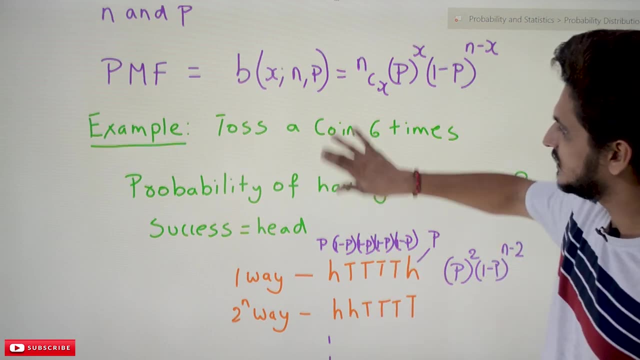 We are tossing a coin 6 times. They are asking a question like this: Probability of having 2 success? Here, success means head, So this is one of the way we are getting success. So success is equal to head. What is the probability of getting success? 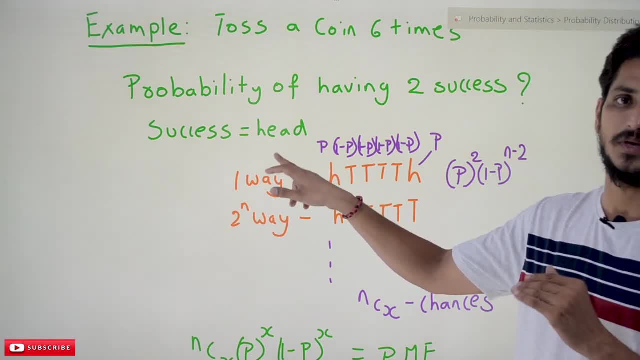 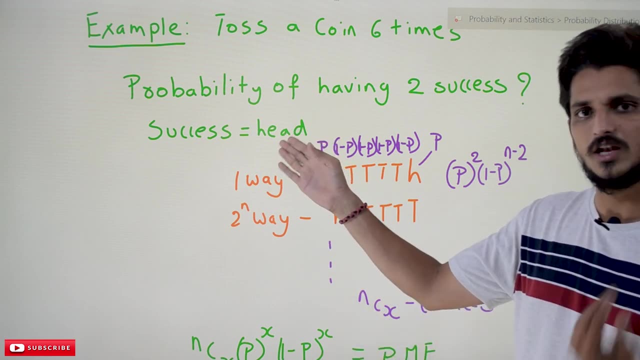 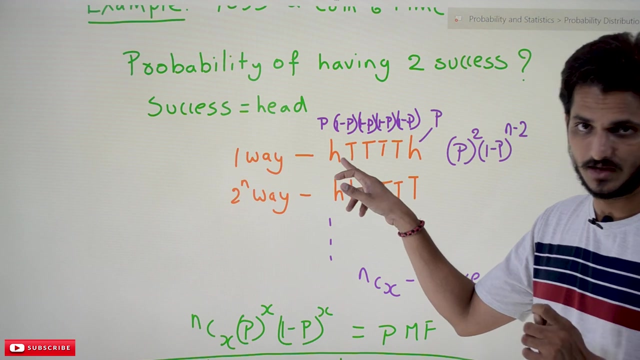 p. What is the probability of getting failure? 1 minus p, Because this is the concept from Bernoulli experiment. If success is p means other option is failure. Failure is 1 minus p. So the first way is when you toss the coin first time, you may get head, you may get tail. 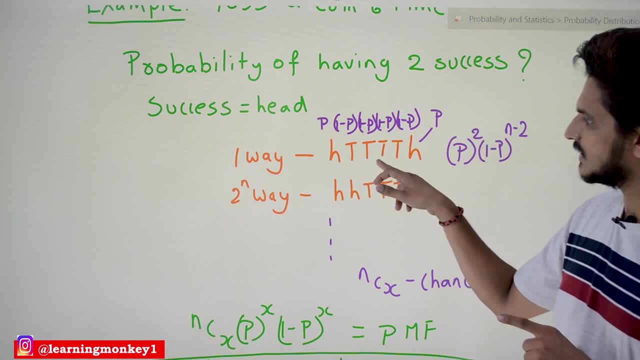 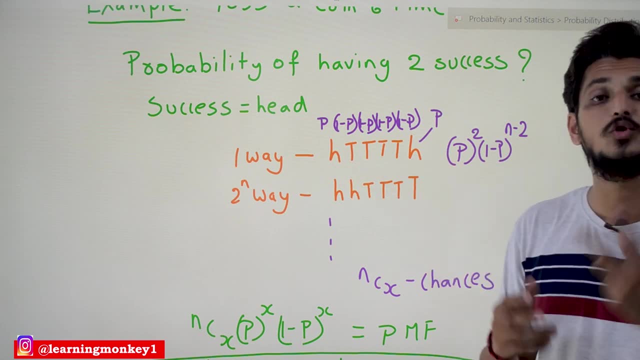 Suppose, if you got head Second time, you got tail. Third time you got tail. Fourth time you got tail. Fifth time you got tail. Fifth time you got head. Yes, this is one way you got 2 success Out of 6, probability of having 2 success. 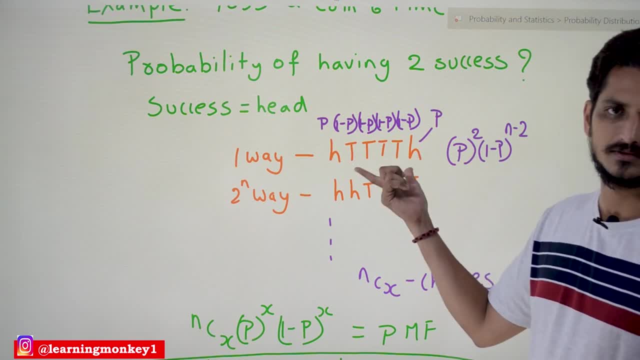 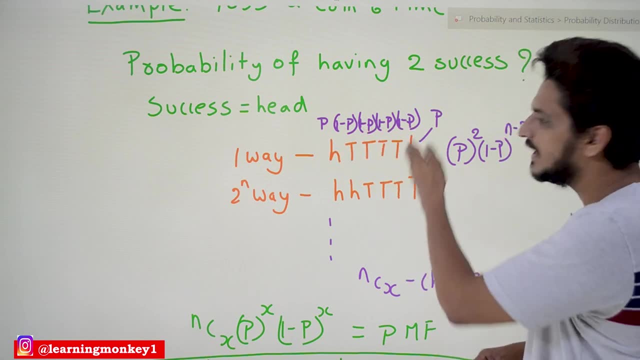 Success is head, So we are having 2 heads. This is one of the way How we find, How we find the probability of this value. All these trials are independent. When it is independent of each experiment is independent How we find the probability values. 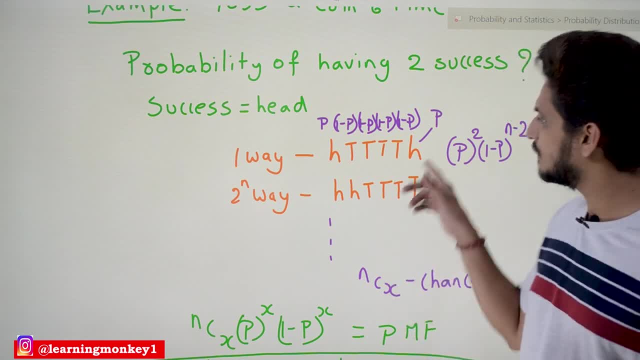 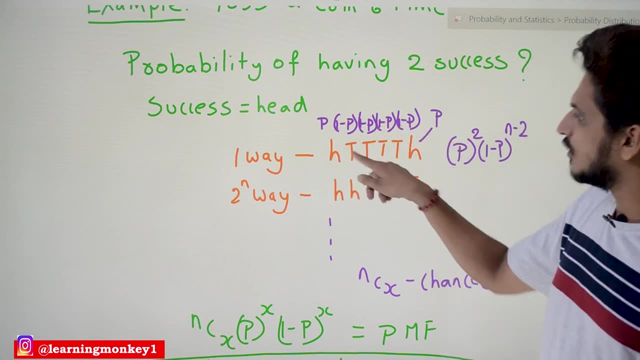 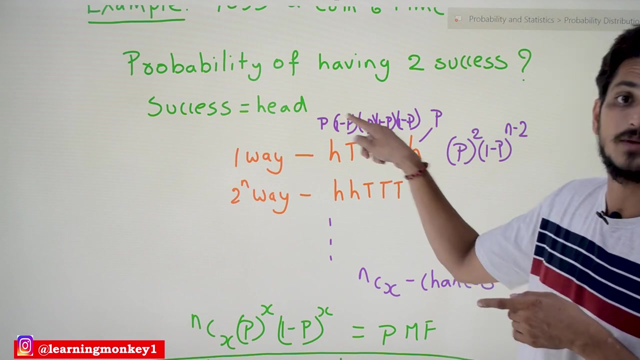 Multiplication theorem in our independent events. Multiply all the probabilities that we, all the values you got from this independent values. That is what the probability value. So what's the probability that you are going to get? head is p, What the probability value that you are going to get tail is 1 minus p. 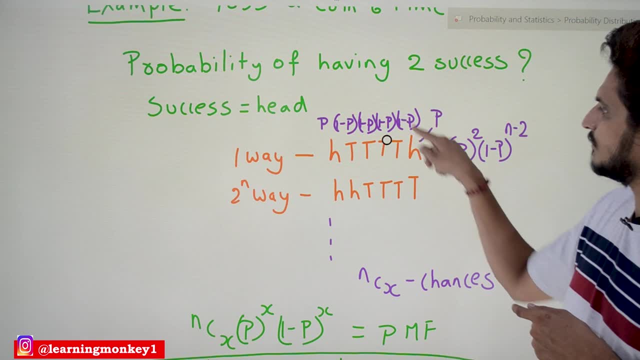 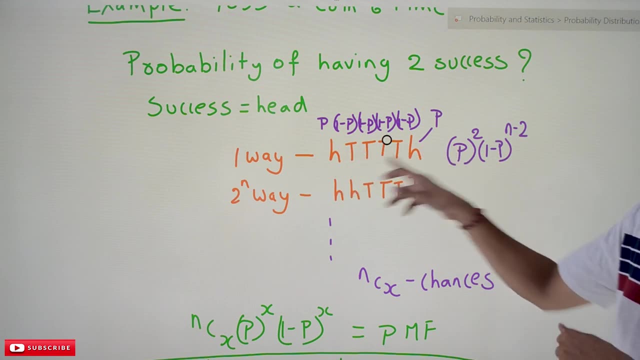 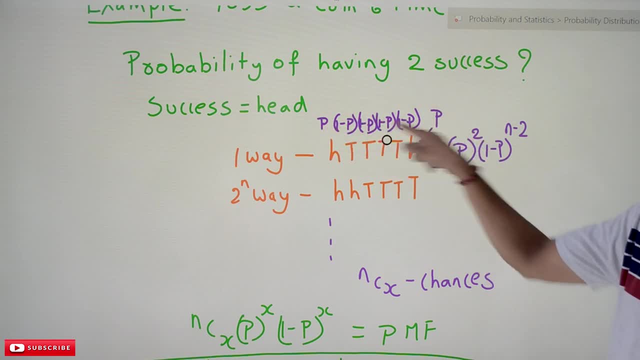 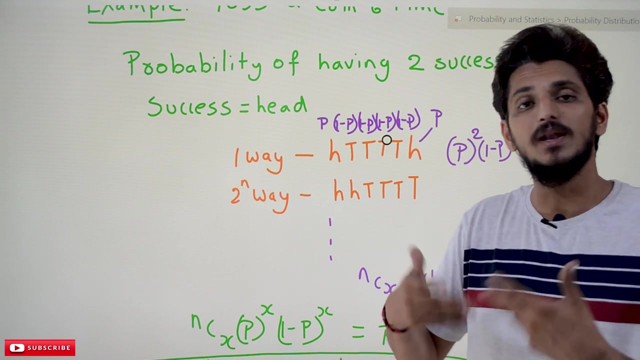 Total n experiments out of 2 are success. remaining are failure. So we are finding the. this is the value you got for this event, But is this the only event that is going to happen with 2 heads? No, there are multiple events are there. 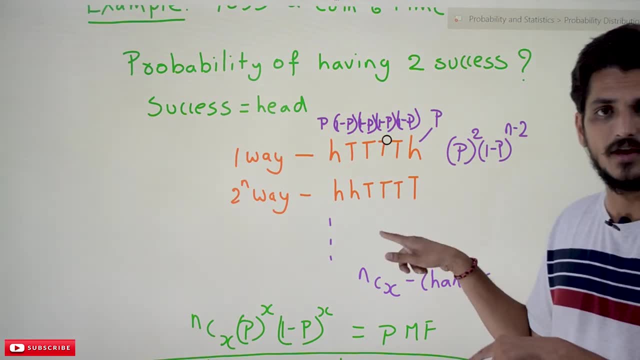 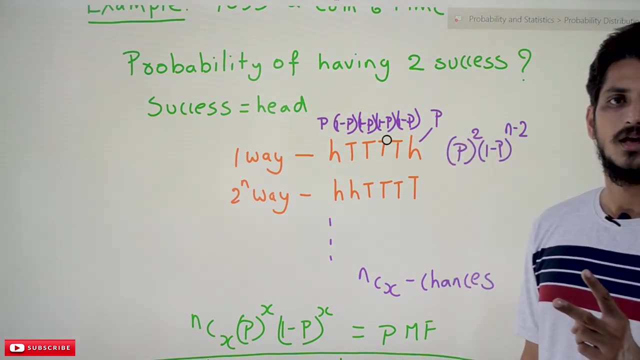 Head, head, tail, tail, tail, tail. This is second way. Like that, how many ways you are going to get 2 success in 6 experiments? This you will get from combinations, The combinations examples which we have done in our previous classes. 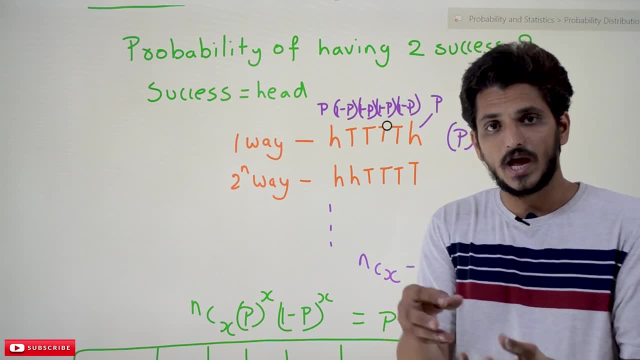 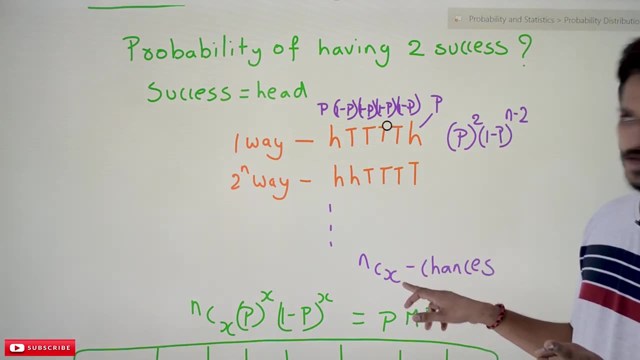 N experiments has been done. out of that you should have 2 success. That is given as ncx, X is 2.. 2 success N means number of experiments we have done: Bernoulli experiments. Here n is 6.. 6 is 2.. 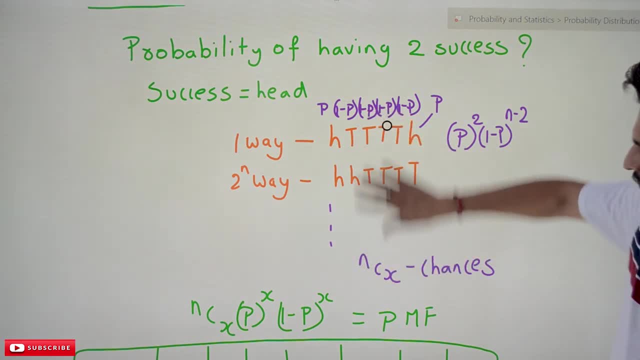 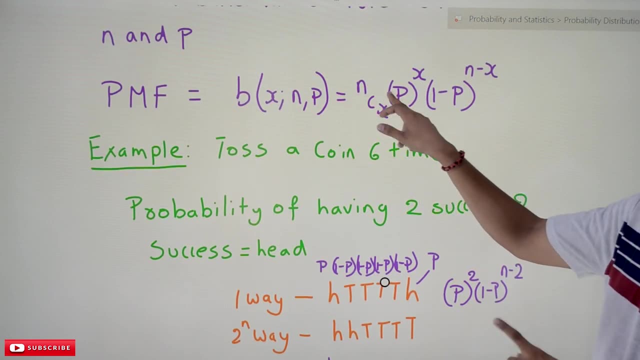 That's why our total, total- we are having these possibilities, We are having ncx- possibilities are there. That's why we got the equation: probability mass function ncx multiplied by p, power x. X is 2 here, N is 6 here. 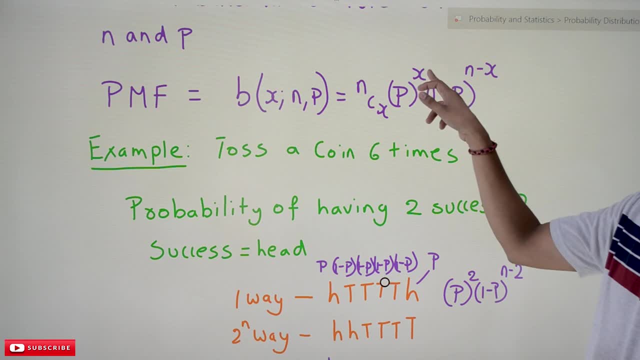 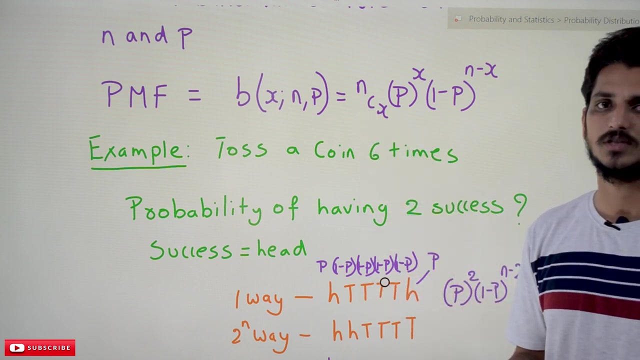 1 minus p power, n minus x X success, N minus x failures. That's why the probability mass function is decided. This is how we got this probability mass function. Until now, we didn't understand what's binomial distribution means. With this probability mass function, we are going to understand what's probability mass function. 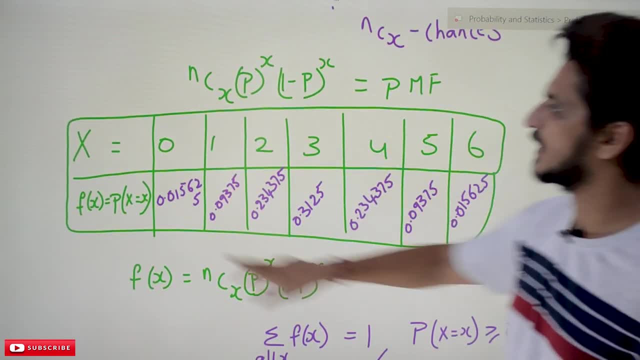 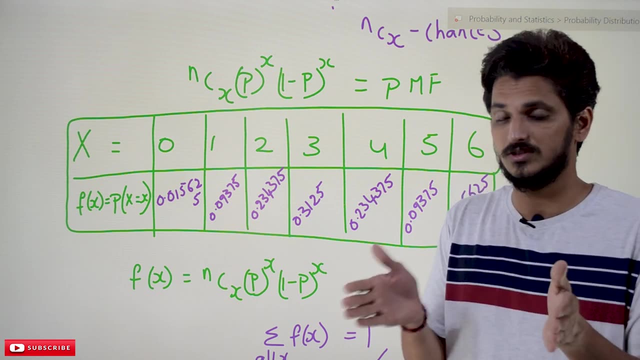 What is binomial distribution? means Now coming to our random variable x. When you toss the coin 6 times means we have done 6 experiments, 6 Bernoulli experiments. What is the possibility of getting 2 heads? What is the possibility of getting 4 heads? 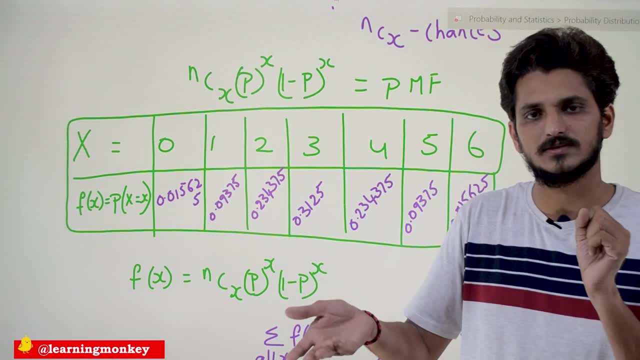 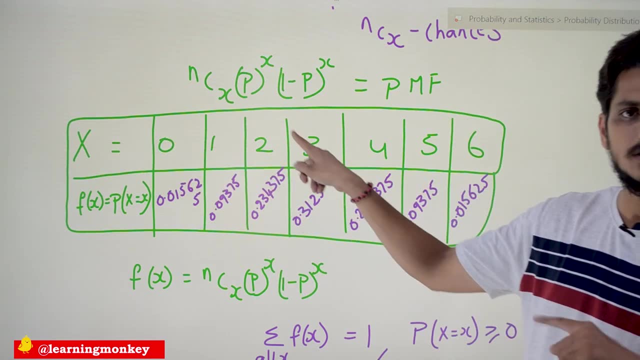 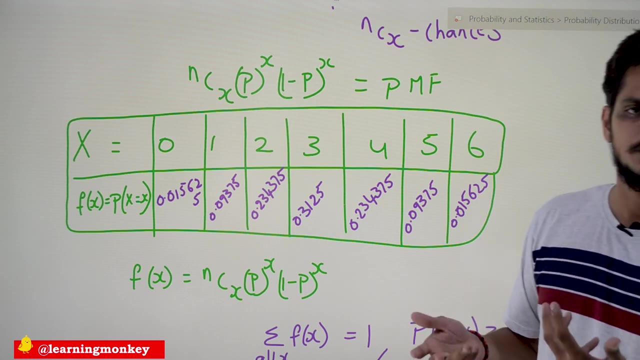 What is the possibility of getting 5 heads, 5 success, 0 success. So our random variable will take: 0 success, 1 success, 2 success, 3 success, 4 success, 5 success, 6 success. 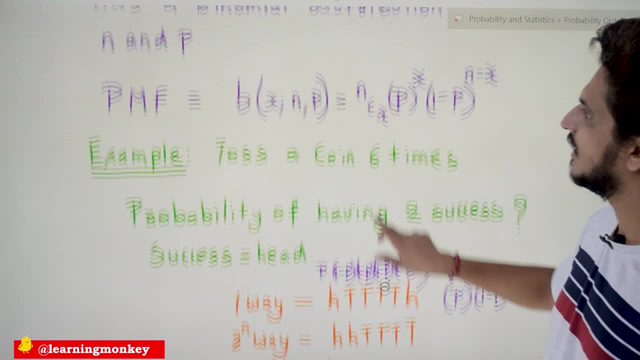 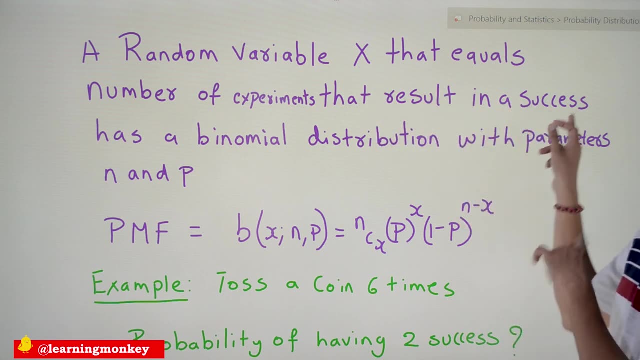 This is what they have given the statement A random variable x that equals number of experiments that results in a success has a binomial distribution with parameters n and p. This is given as b of this is the formulation which we use it for binomial distribution. 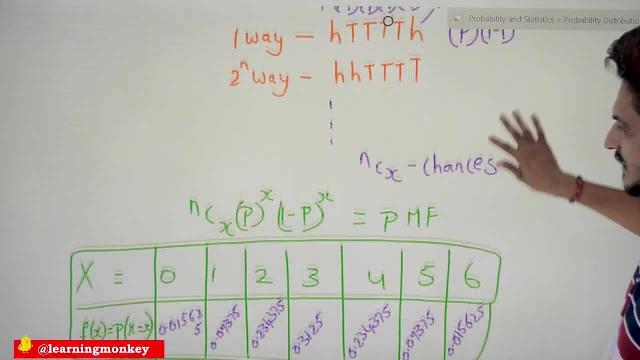 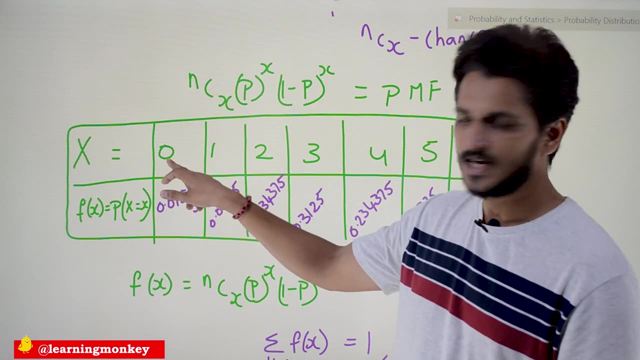 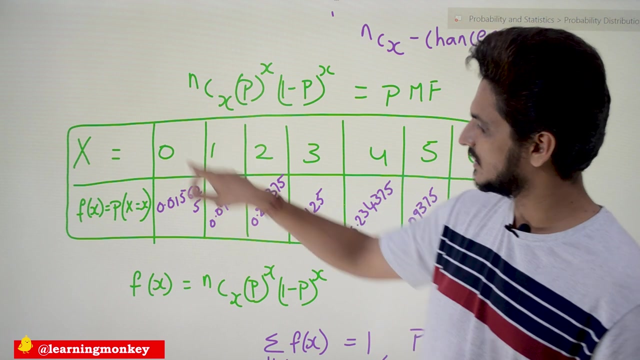 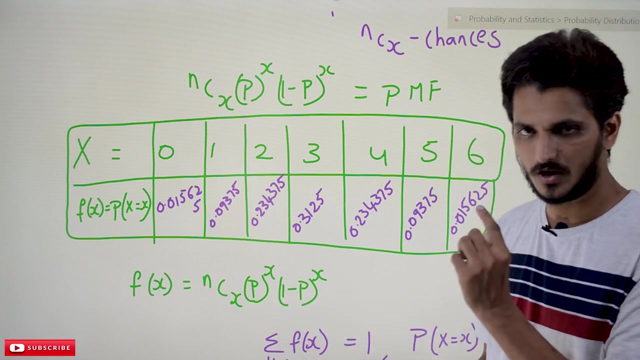 The probability mass function is this. Now, coming to our example, this is what the probability distribution means. Binomial distribution means 0 success. Success can be identified by f of x is equal to f of x means probability mass function. Probability of x is equal to x is a small. x is taken as 0, n c, 0. here n is 6, 6 c 0. p means probability of success. power of x: 1 minus p. power of x. 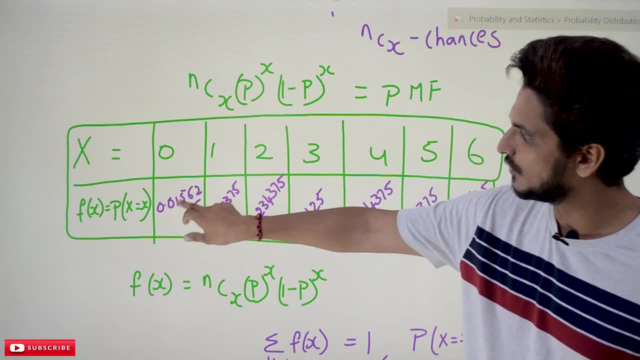 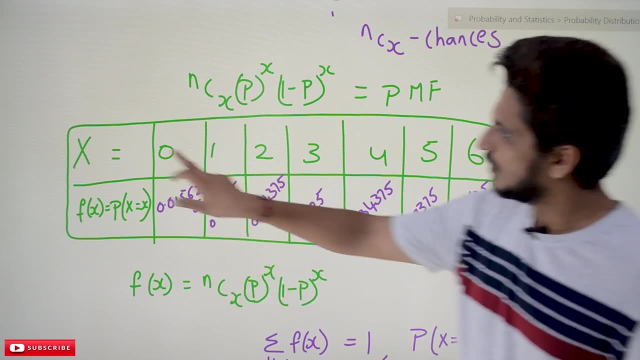 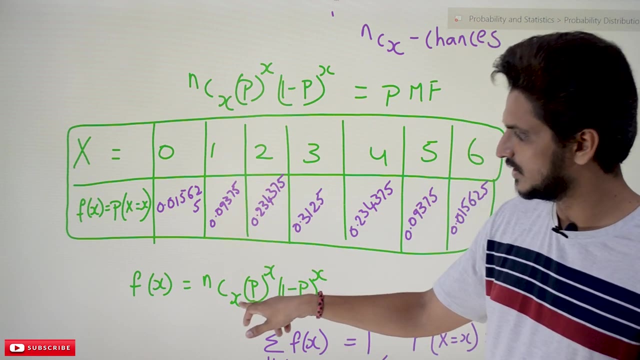 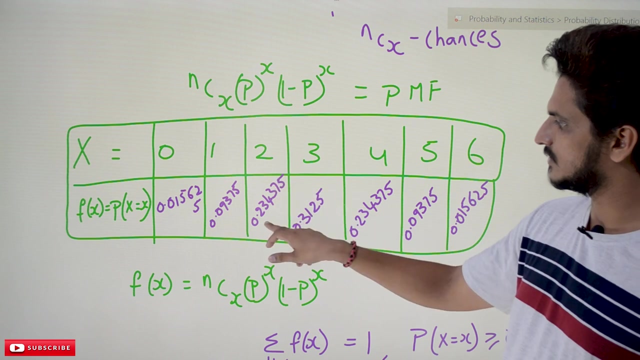 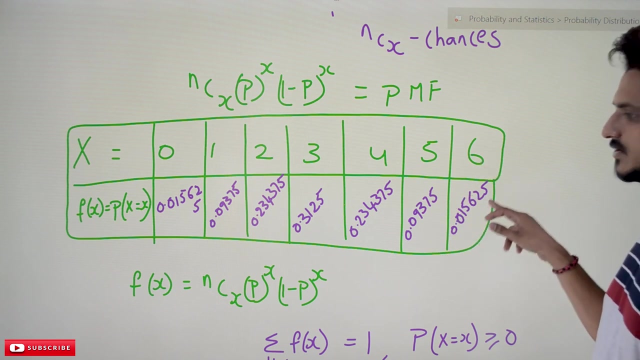 If you substitute this in the in this equation, we got this value 0.015625. we are not doing the calculation, So this is the value. So x is equal to 1 means 1 success out of 6 experiments: 1 success. this is the value you got. if you substitute 1 in this equation, n is a, 6, x is 1. we got this value 0.09375. 2 success. this is the value: 3- success. this is the value 4- success. this is the value 5: success. this is the value 6: success. this is the value. this is what binomial distribution means. 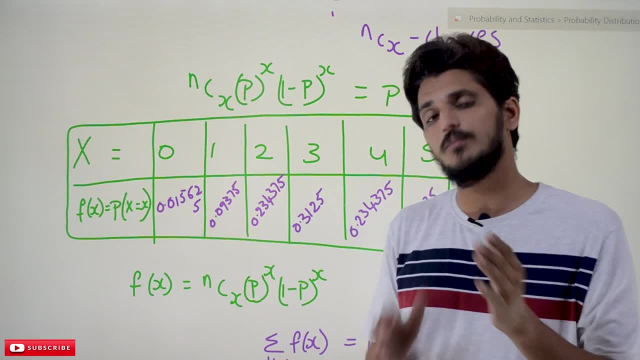 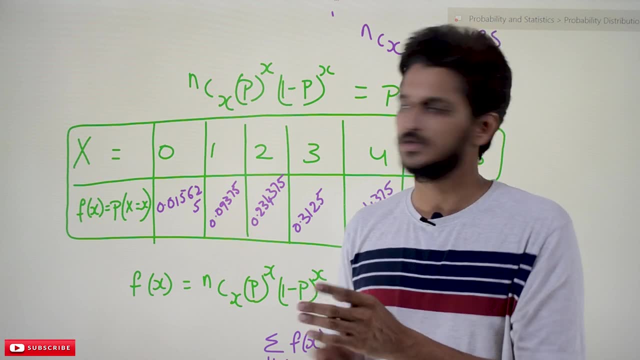 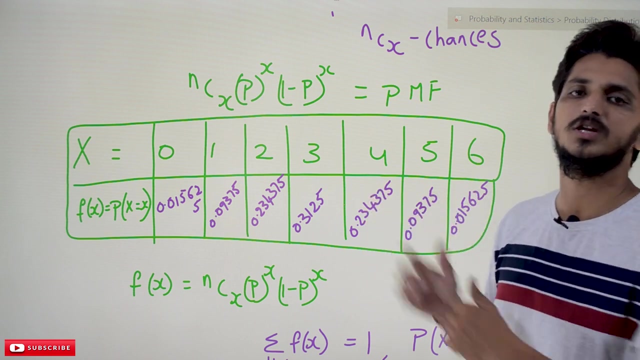 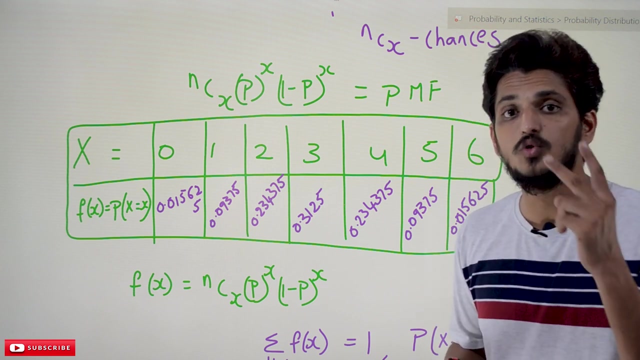 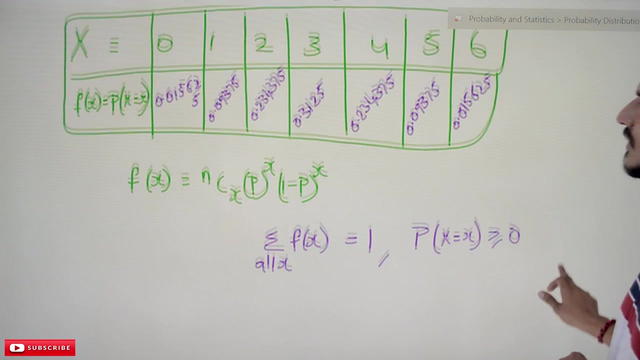 So in our last classes, when we discussed about problems, Probability distributions, distributions, two types of distributions are there: discrete and random continuous distributions. this comes under discrete distribution. binomial distribution is a discrete probability distribution. So in order to obtain probability discrete probability distribution, you should follow two conditions. what are those conditions? probability of x is equal to x should be always greater than or equal to 0. 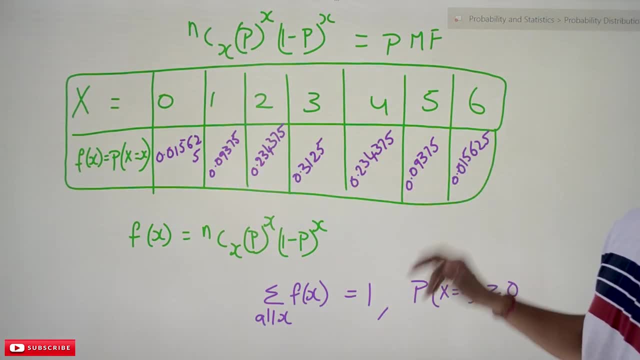 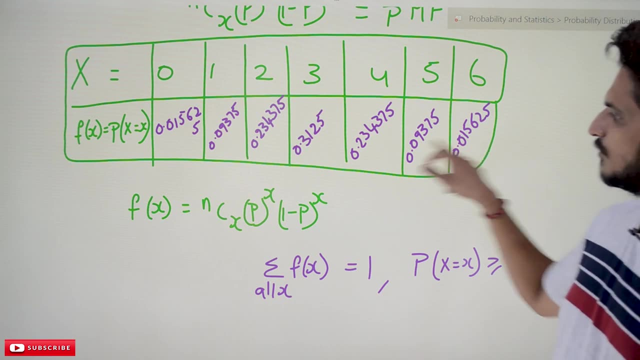 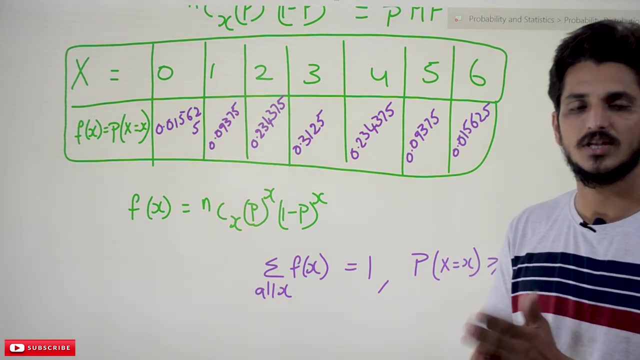 Yes, So the probability of x is greater than or equal to greater than or equal to 0 and summation of all this problem probability should be 1. if you summation of all these values, probability values, we will get 1. yes, it is following our probability distribution conditions. discrete probability distribution conditions. 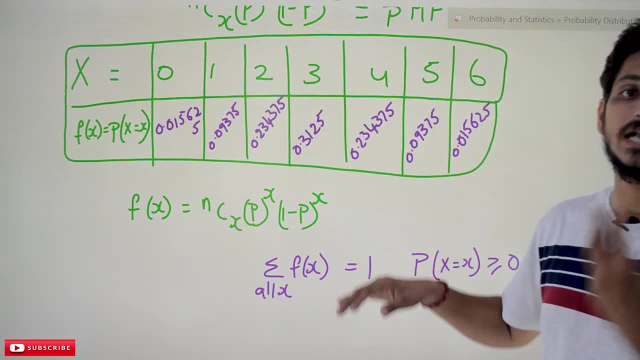 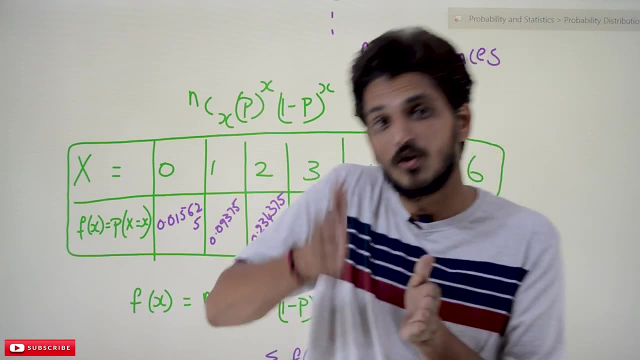 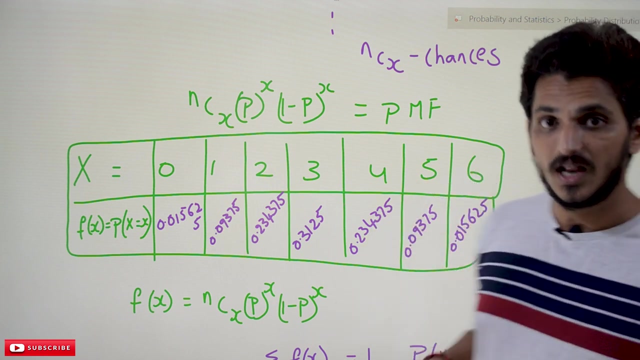 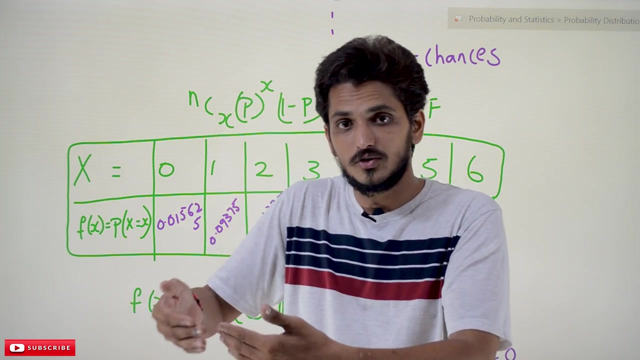 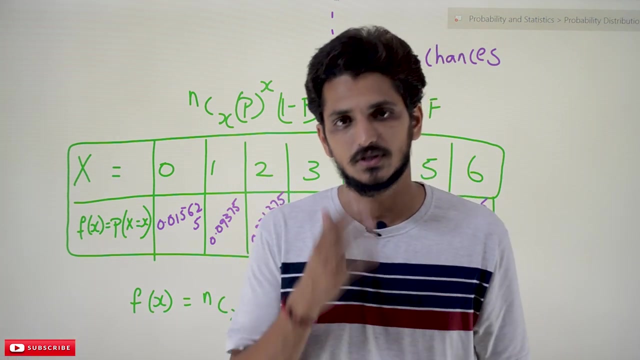 So that's why this is this is what. in this type of situations, we can apply binomial distribution. So what's the type of situations When repeated Bernoulli experiments are done? we can take that success values into binomial distribution. the real life examples and data analysis examples will be discussed in our coming classes. with the data analysis example, we are going to understand Poisson distribution also. if you have any questions regarding this concept, please post your questions in the comment section below. thanks for watching. if you haven't subscribed to our channel, please subscribe to our channel and press bell icon for the latest updates. Thank you.